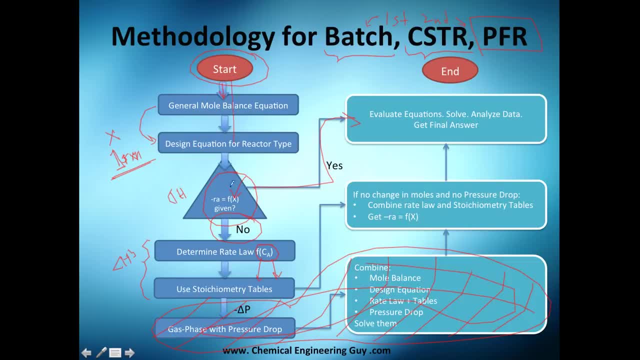 And yeah, essentially we're going to follow this path here and then go here. We need to combine the rate law with stoichiometry tables. So what we do here is Q. we do very well with stoichiometry tables. So if this period, for example, is negative, it should be negative. 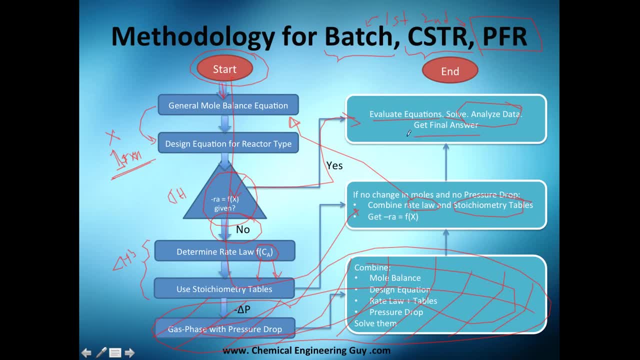 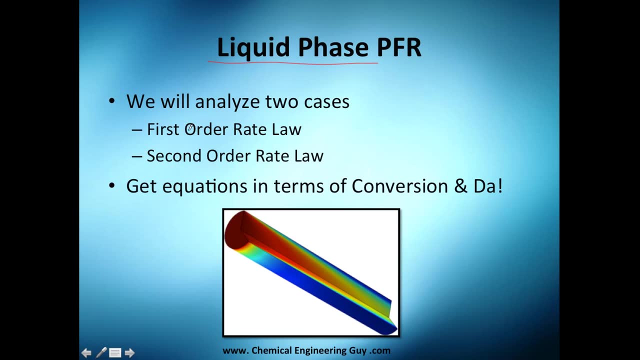 Now cut to the solution of our equation. So what we're going to gonna do now is we gotta calculate our design equation. So once we do that, we evaluate the equations we solve for the problem and, of course, analyze your answer and get your final answer. 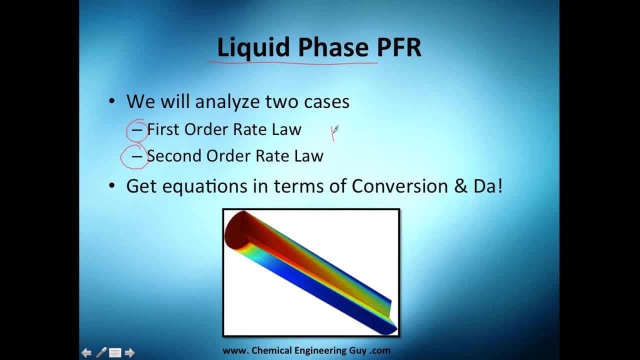 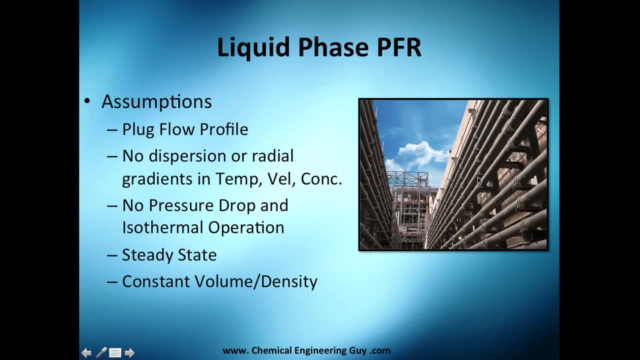 Now let's talk about the liquid phase P. We will analyze two cases. I told you before the first order and the second order. we need to get the equations in terms of conversion and, if possible, the damp color number Assumptions of the liquid phase P. well, you have, plug flow. 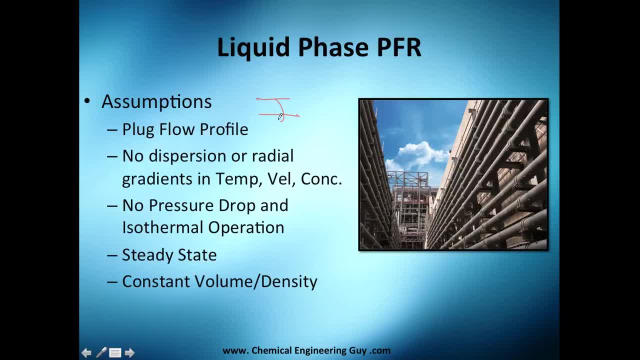 profile. so instead of having this here like the normal profile, typical curved side- you have almost zero speed here and highest point here we have a plug. so all the profile is like this. When is this possible? When you are super turbulent or your stream is super turbulent. Now we have no dispersion on radial gradient, so 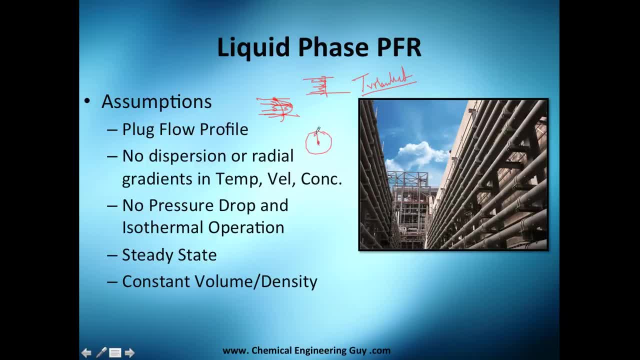 let's say, temperature doesn't change if you're in the center or in the wall near the whorl. and the velocity also we have. I told you before we doesn't depend on the radius and the concentration doesn't change. Now we have not pressure drop and 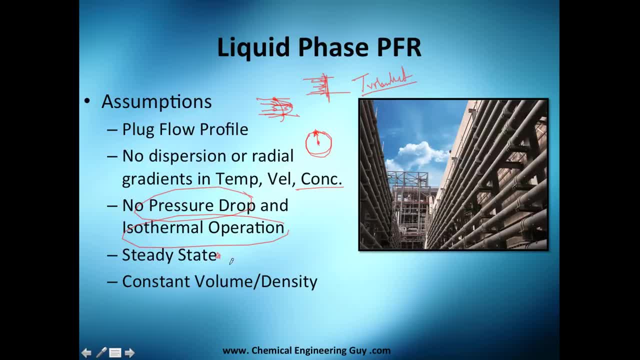 the concentration doesn't change. We have no pressure drop and the concentration doesn't change. Now we have no pressure drop and it's isothermal operation, of course, is a steady state because it's a PFR continuous reactor and we have constant volume over density. I think the that's 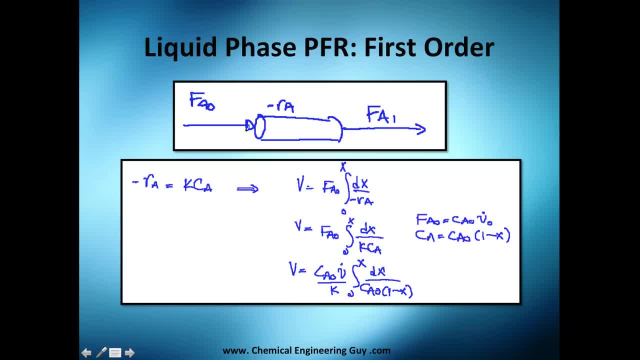 the main difference with the gases or the gas phase, PFR. Now I remind you: how is the reactor? you have an inlet, you have an outlet, you have a rate of reaction, you have probably a conversion and your reaction. So let's start with the rate of reaction of first order. you have your 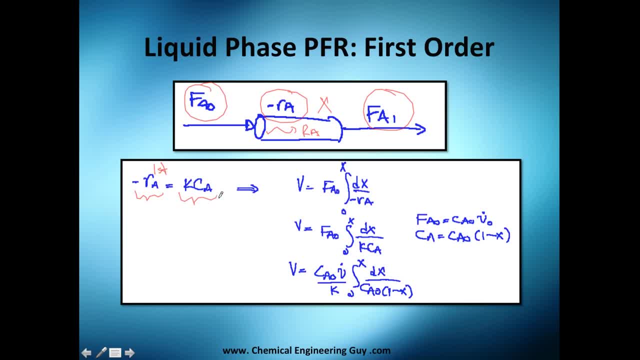 rate of reaction here and by definition it's the constant times, the concentration. Now, this one here is our design equation. it does not depends on the rate. so if it is first order or second order, this is still our design equation. If you don't have any idea where we got this, go back to chapter 2. 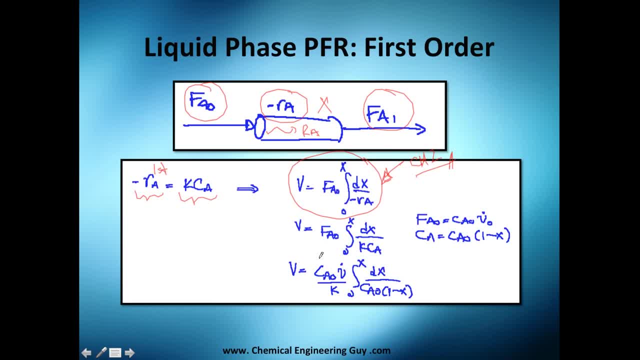 we got that in that topic. Now the first thing I want to do is to substitute this value here with this one here. So I got it here. you can see everything. the flow of A at the beginning is just here, outside the integral, the x here. okay, Now. 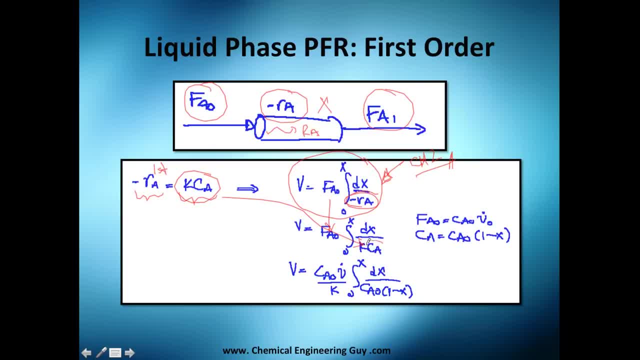 I'm going to do two things. first thing of all, I want to change this concentration in terms of conversion. I use this formula here. remember the initial concentration and the difference of conversion. This is a constant, so your new variable will be conversion. But not only that. I want to change this right. 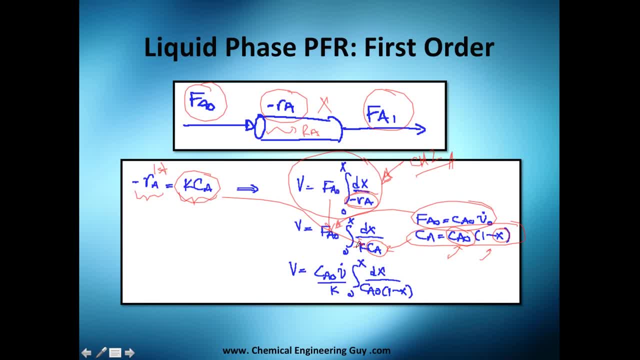 here, my flow. So I got this. the k is a constant. I can take it out. the volumetric flow stays here, the constant here, and I have this here. You will see that the constant. actually I just jumped this, but, as you can see, this is a. 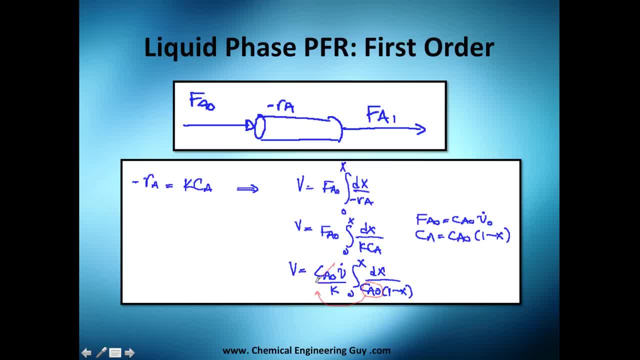 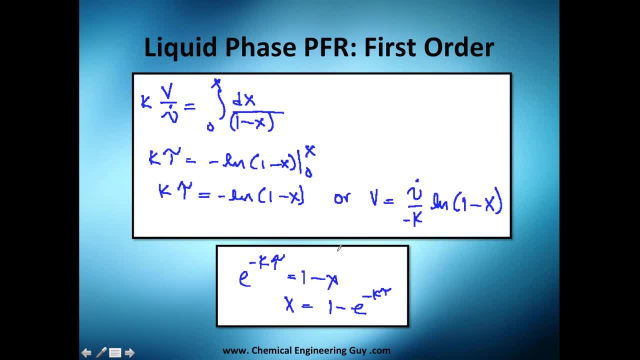 constant so I can take it out. And it's the same constant here, I can take it away. So I'm left with volumetric flow rate and the constant. But not only that, I send them to the left so I can have my integral alone here. Now, by definition, this part right here is the space time. 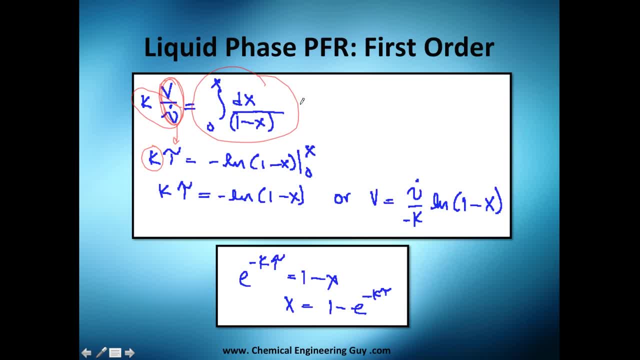 here, My k is here and I solve this with a table of integrals. So it's essentially just the negative logarithm of this part right here And I need to evaluate from 0 to X. Once again, I do this, you know this, you will get that. 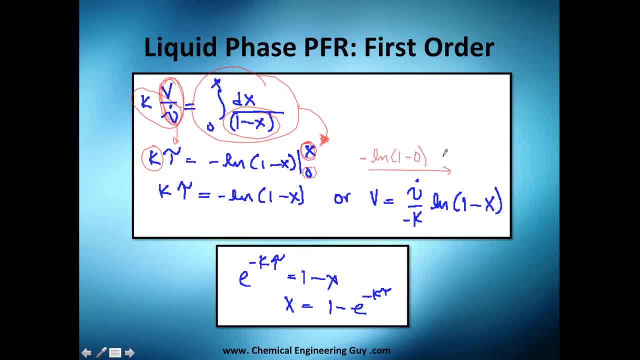 This thing right here. check it in your calculator. the logarithm of 1 is 0, so actually you could just ignore this part. Mathematically is this part right here. Or if we want volume we can get like here. I really prefer this one. 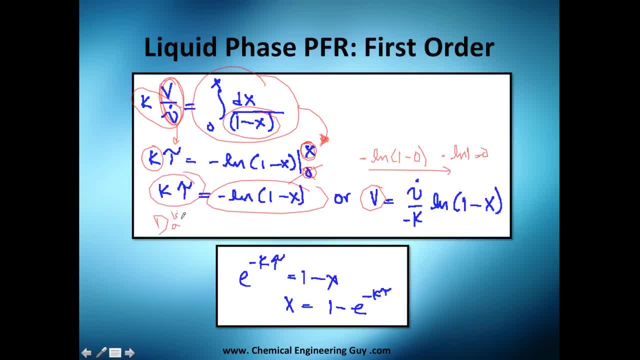 because we're going to play with it. It's actually the damped color number for a first order differential equation, And if you wanted to solve for X, you get this, This part, right here. X equals 1 minus the exponential of minus k tau. Now, that was first order. We are going to. 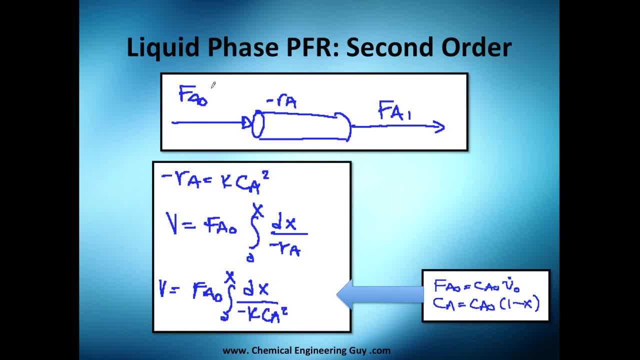 analyze later. Now, second order: PFR in liquid phase will be the same. You have the same inlet outlet reaction, but this time is second order. What does the second order means? It means that it depends to the second power. here Now my volume equals this part. Exactly the same process, but I substitute here the concentration. 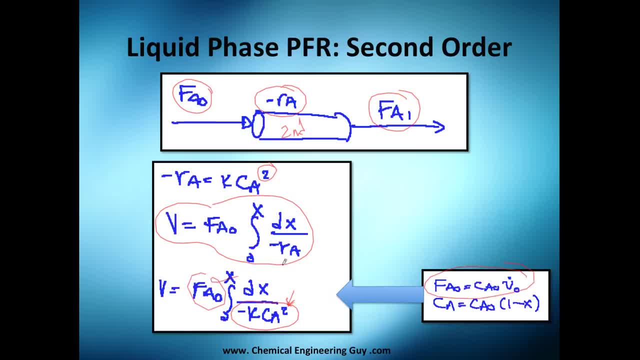 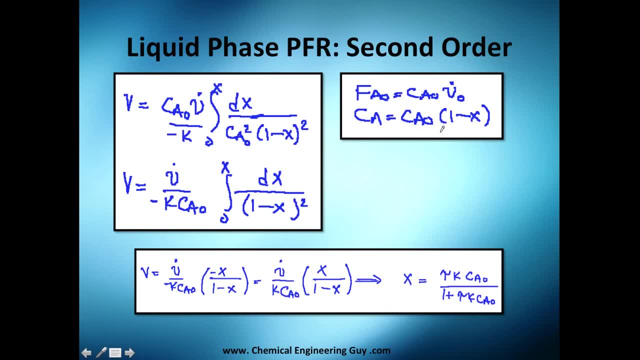 to the square. I will substitute the same data here as I did before. Also, concentration: I need to change it into conversion And the thing here is that I have to the square, so that's why I have to the square to the square here. I substitute this data here, Remember. 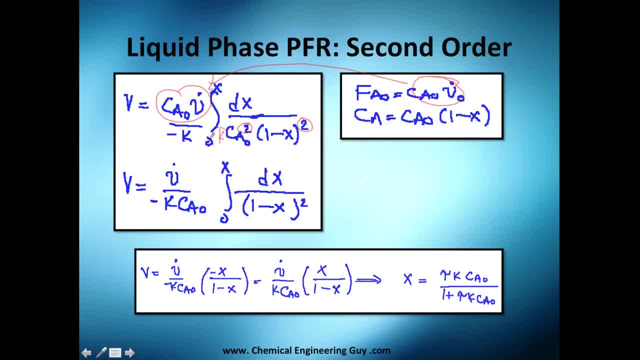 the K was supposed to be here, but I'm just taking it out and I get this: The concentration is to the square. so when I take it out, I will get concentration to the square, and this is only to the first power. so this goes out, and this too goes out. That's why, as you can see, 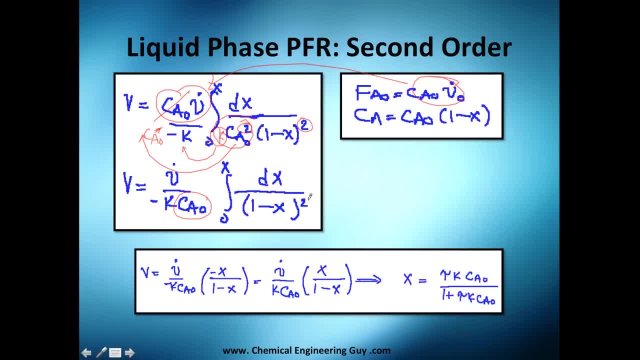 it now depends on the initial concentration. Now, let me solve this. I used a, let's say, a table of integrals. I got this. As you can see, this is the solution of that integral. and then what else I did? well, okay, take out the negative sign here. okay, and I just solved. 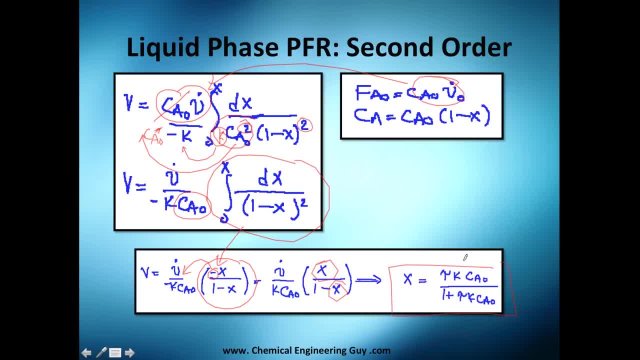 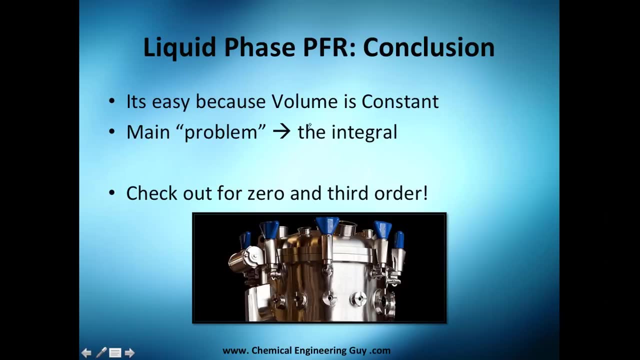 for x. It's easy and I got this equation. So, as you can see, we have still the tau times k, tau times k and the concentration. So what's the conclusion on this liquid phase PFR? Well, it is easy because the volume is constant, So playing with the integral is not that much. 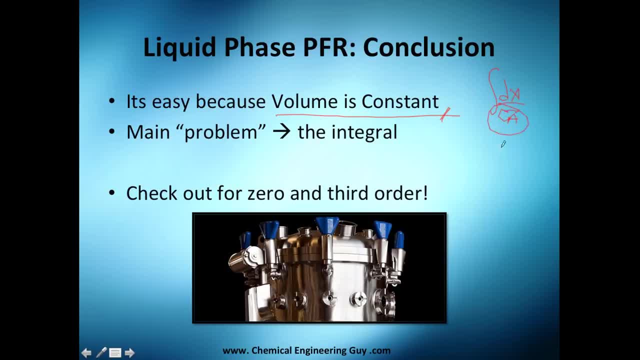 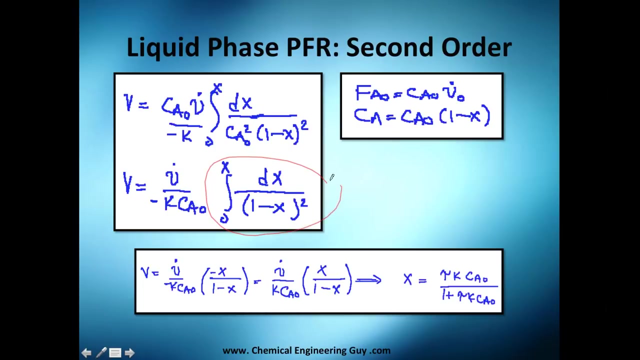 problems, and especially concentrations, since the concentrations have constant volumes. so you know, concentration is actually moles per volume and this volume is constant. we can actually do easy mathematical processes. The only problem that I see is the integral. So let me go back This thing. maybe you don't know how to solve it, or if you are in the 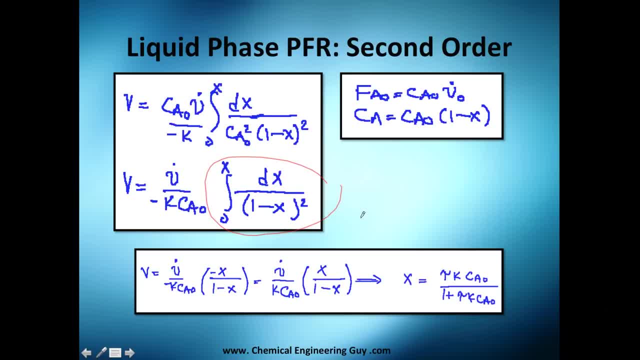 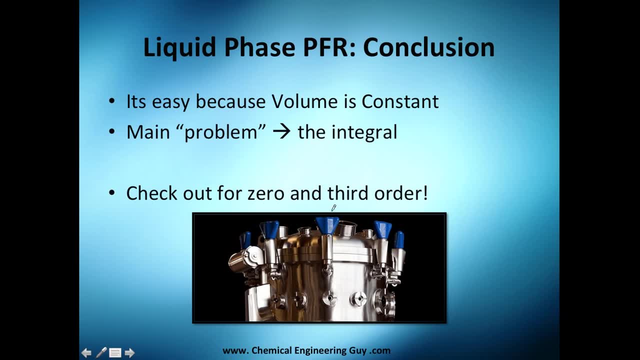 exam, you get blocked or you have no idea how to solve it. well, that's only mathematics, It's no problem, and I think many calculators can actually solve that. So I think the worst part is the integral, And if I were you guys, I'm not going to show it, but or maybe I show. 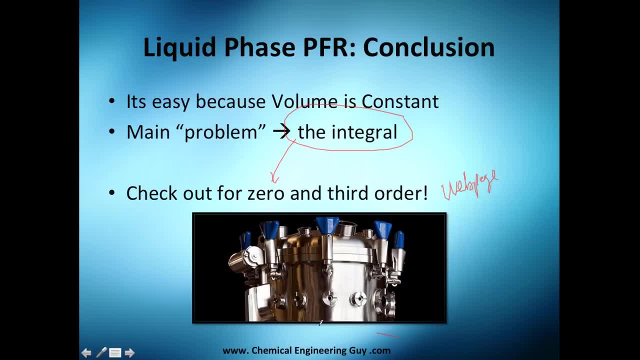 it in the web page. Web page here. Go here to courses, chemical engineering- and then go to reactor engineering. Check it for zero, it will. it should be easier. and third, it's a little bit more complex but still easy because of the concentration being, or having a constant volume. I'm not going. 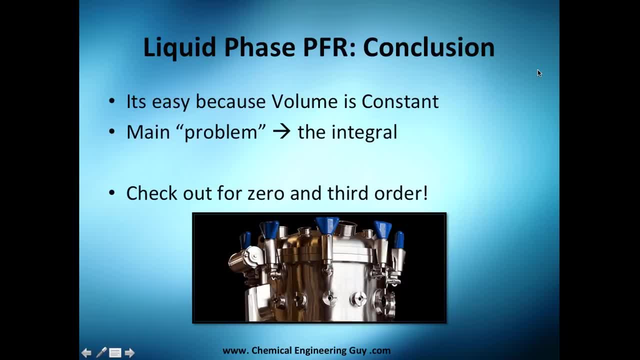 to solve. yeah, I'm not going to solve any problems because this is as we did before in chapter two. It's not that different at all. The interesting part is when we start analyzing gas phase PFRs. So once again, you need some problems, probably you will find. 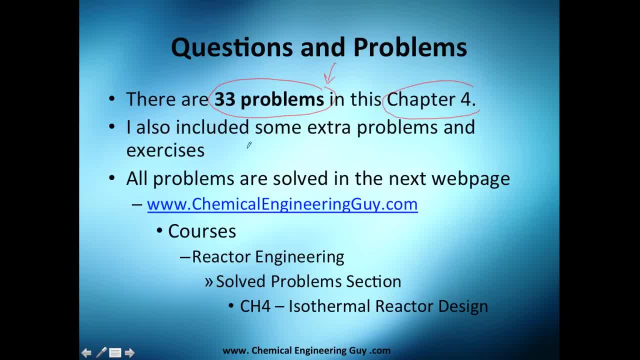 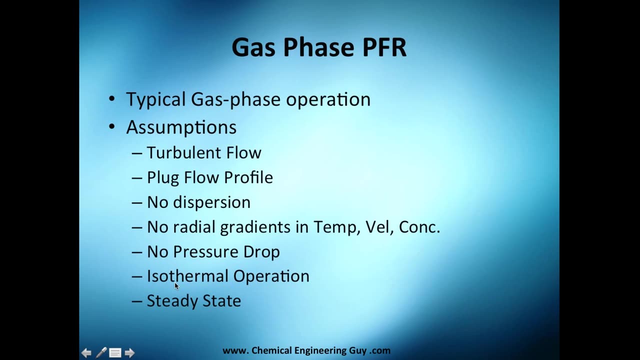 them here. in the back of this chapter four, I also included some extra problems and exercises. you want to check them? Just go to my web page courses- reactor engineering- solve problems and you will find everything in here. So the next one will be gas phase PFRs. 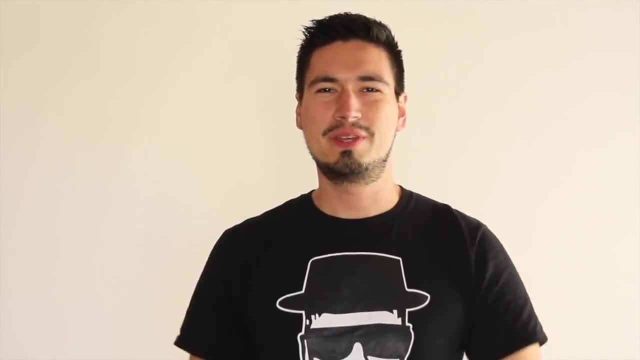 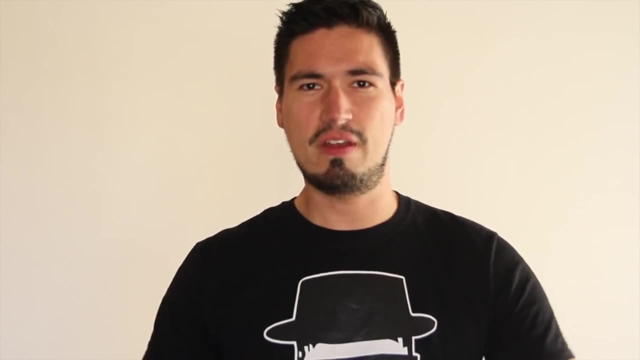 What's up guys? it's me chemical engineering guy. So if you like the video, why not push the like button? It really helps me to know if you're liking the videos or if I should be changing something or I should be adding something, taking out content, whatever. Also. 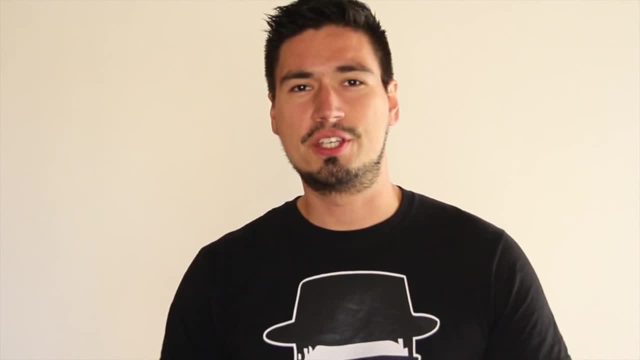 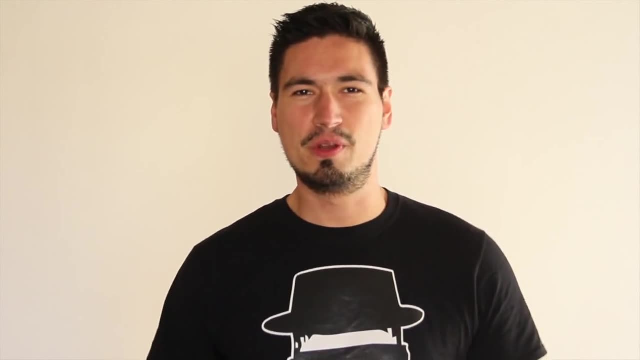 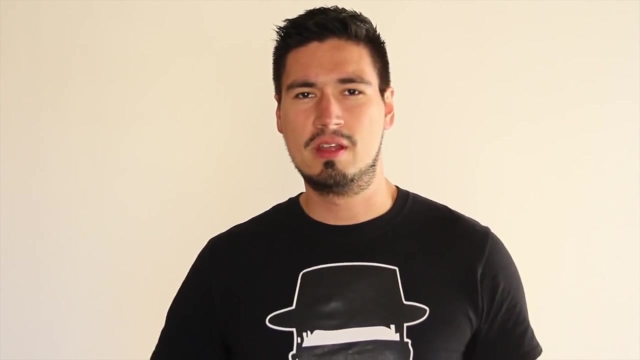 sharing is caring, So if you got any kind of friends, teachers, colleagues or whatever kind of person that might be interested in this type of content, why not share it? Sharing helps our community to grow faster- in members and in content. If you want to keep track of my activity- videos, uploads, experiments, playlists, whatever- 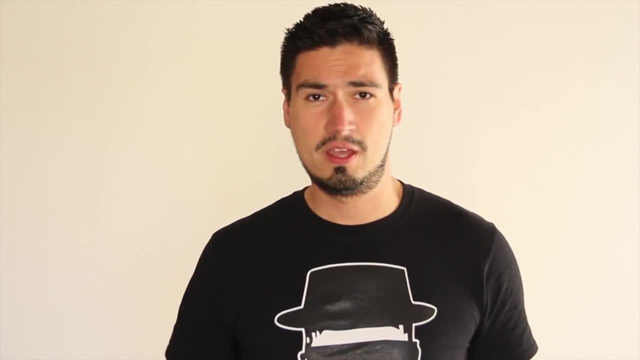 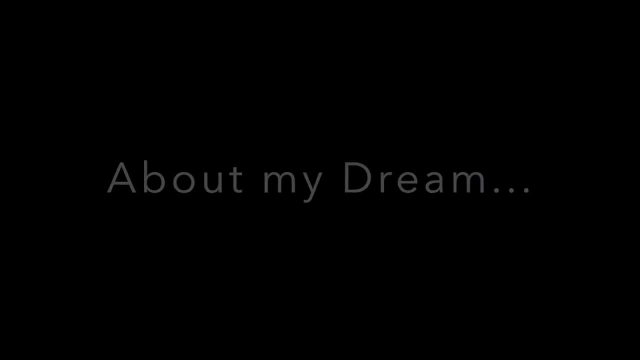 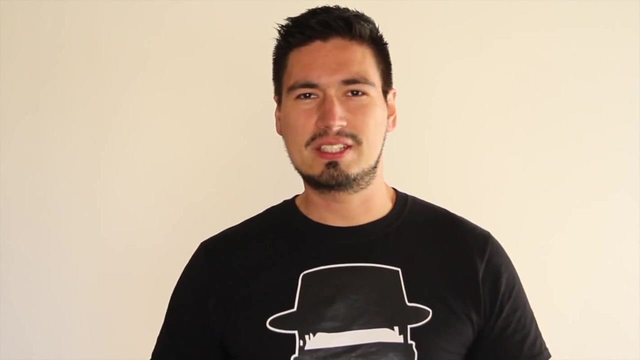 content I'm getting on YouTube. be sure to click the subscribe button. Subscribing to the channel is totally free, guys. My dream is to create an online academy of chemical engineering where everyone can access it in the world. Imagine a place in which the student, the teacher and the engineer 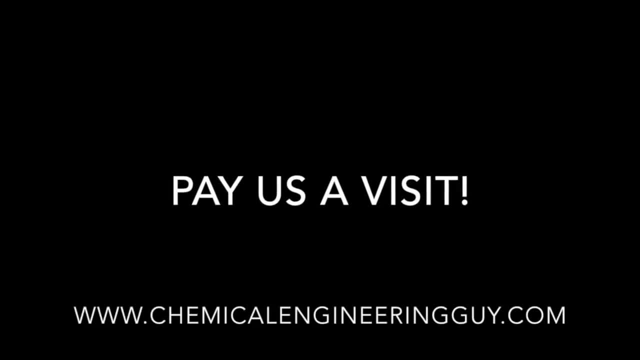 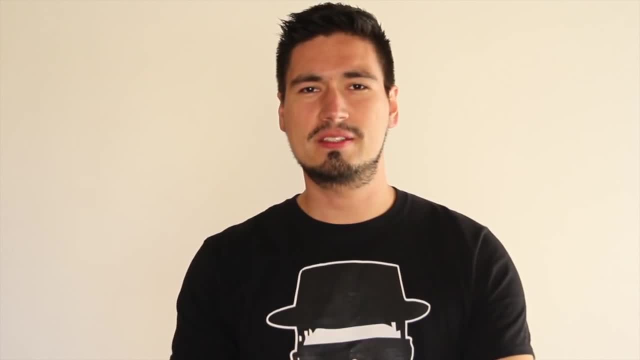 get the best of each other. So thank you, thank you, thank you guys, for the support and the love. 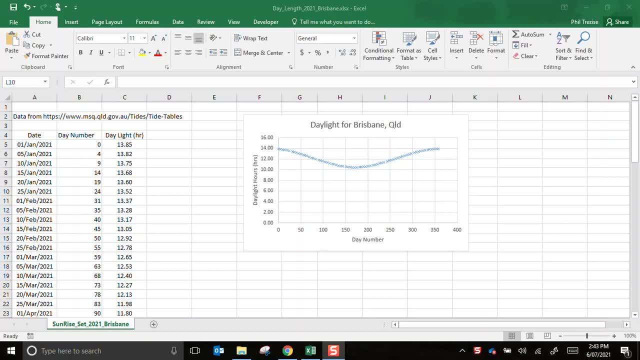 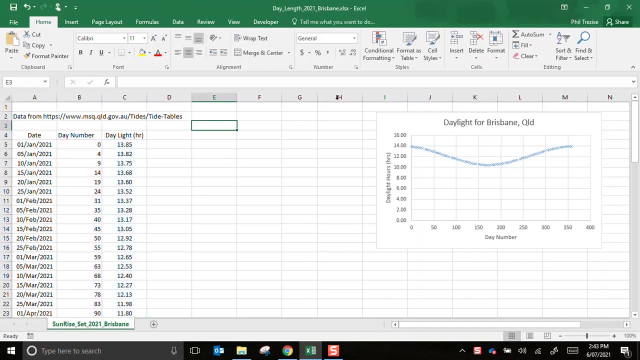 Hi everyone. In this video I'm going to create a mathematical model, a formula, which will do its best to match the data points that we plotted last time. So I'm just going to slide that across a little bit to give myself some room, and I think I will insert a few more rows here. 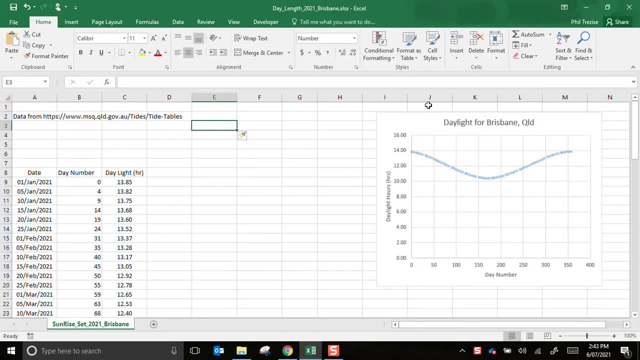 to give myself a little bit more space to work with. That sounds good Now, before I start working on my model. taking a look at this, it looks like some sort of a trigonometric function. It looks like a crest then coming down to a trough and then back up to a crest. So it's a cyclic type of a change and cyclic things. 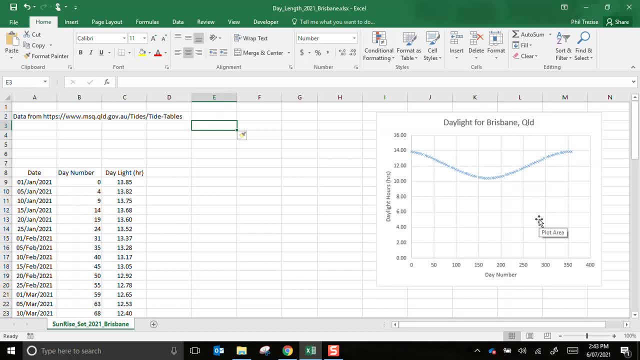 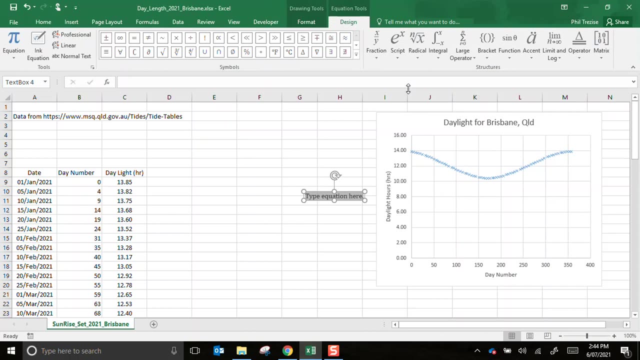 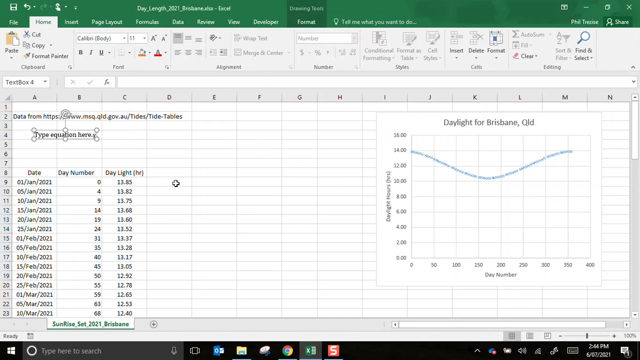 which happen quite often in nature, are often modeled very well by something like a sine or a cosine formula. We call that our model. Now, before I get too detailed, I'm just going to add an equation here. This is just a little reminder and I'll type the equation. 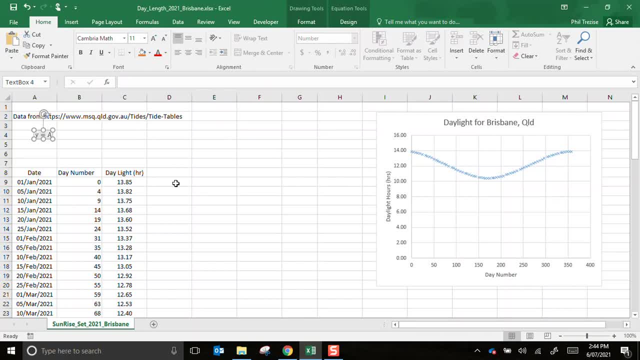 except I missed. Here we go. y equals a by the sine of bx plus c plus d. Now that's a bit small, so I'll increase the size of that a bit and I'll put a little tiny bit of shading behind there. So that's the.